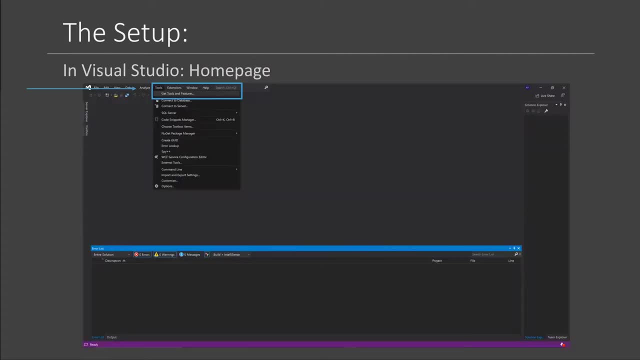 your code. So once Visual Studio has downloaded, we will need to download a tool to allow us to code in C++. On the homepage of Visual Studio, you will need to go to Tools and then click on the Get Tools and Features. Visual Studio will open up this window. 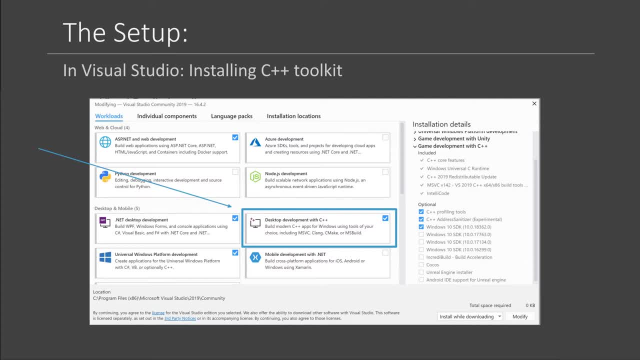 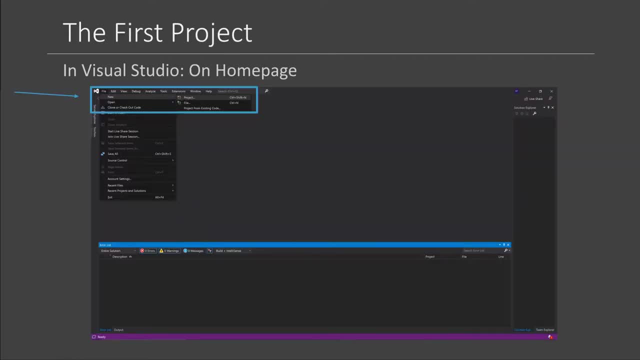 You will need to install this package: Desktop Development with C++. After it is done downloading and installing, we are going to make our very first project. To make a new project, you will need to click on File and then New Project. This will open a window where you will need to select an empty project and make sure it. 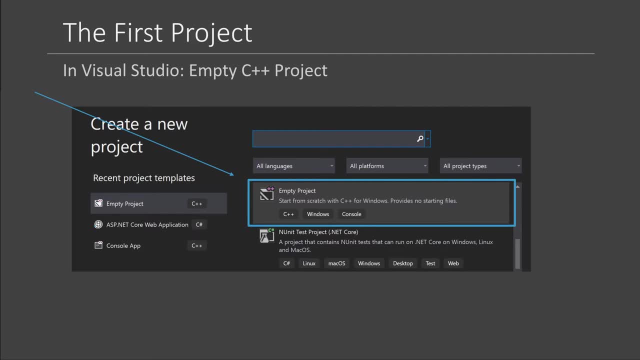 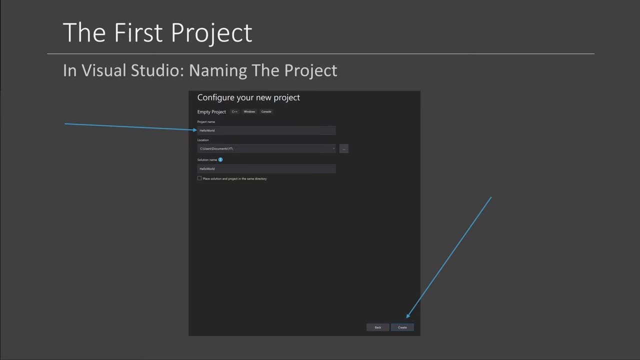 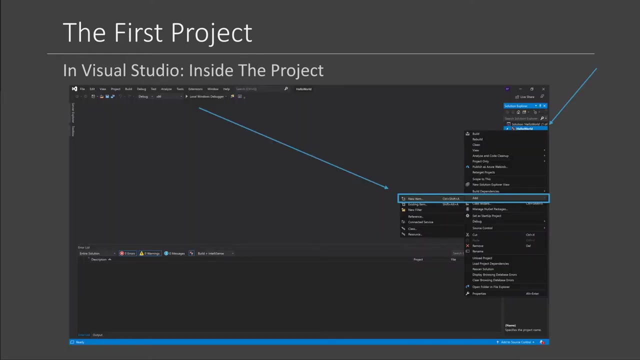 mentions C++. It has to be empty. Now we need to name our project. For the sake of tradition, we will name our first project Hello World. Then click Create Inside our new project. we will left click on the Hello World in the Solution Explorer. 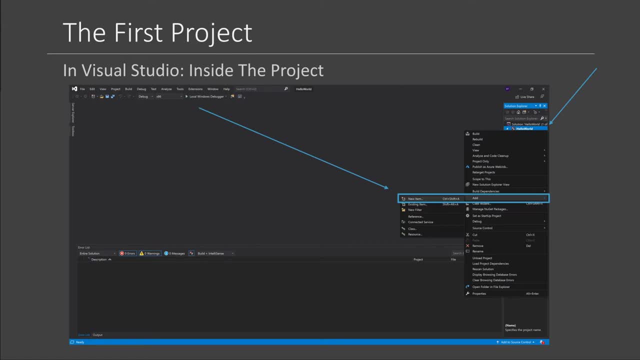 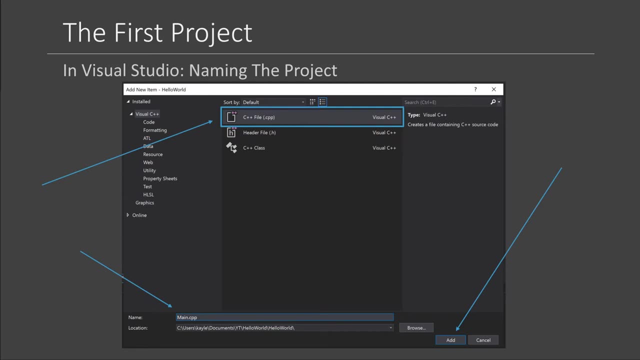 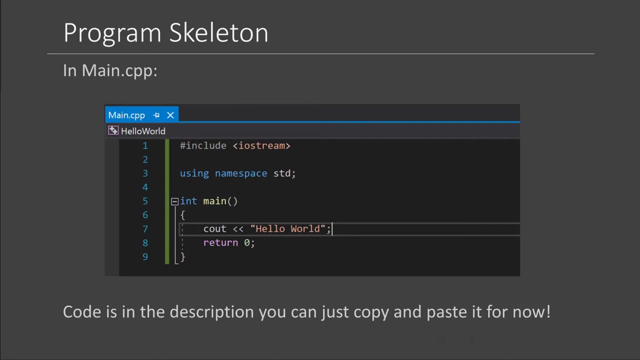 and then Add New Item And then it will open this window where you need to make sure you select a C++ file, name it Main and then click Add. Maincpp will be blank when you first create it. To make a computer do something, we need to provide it with some code. 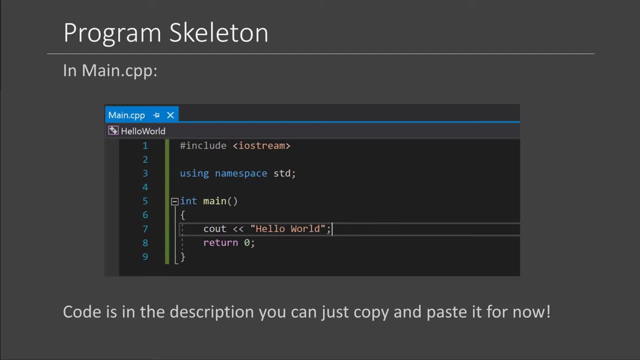 Because we are only starting. I have already typed out the code that you need for this program and I put it in the description box below. So for now, only copy and paste the code into your document. You will learn what everything means in due time. 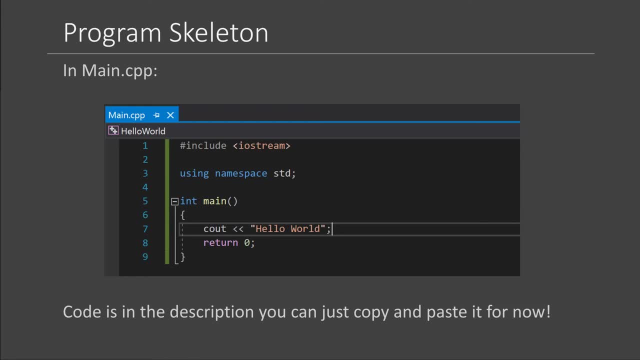 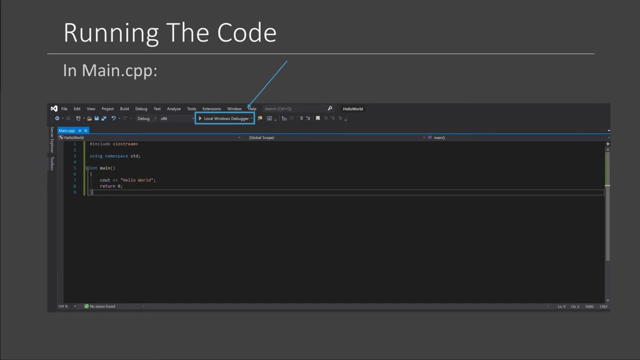 You need to save Maincpp. Now you will find you ready to run your code. Thanks for watching How you run your code. is you want to click on this little green play button and then the compiler will compile your code and then it will produce the following output: 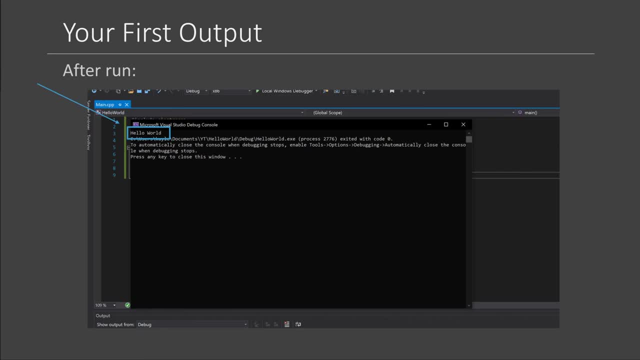 Basically, it will just be a black box with the words Hello World printed on it. This black box we call the console, And then congratulations. this is your first program. I hope to see you in the next lecture and have a nice day.